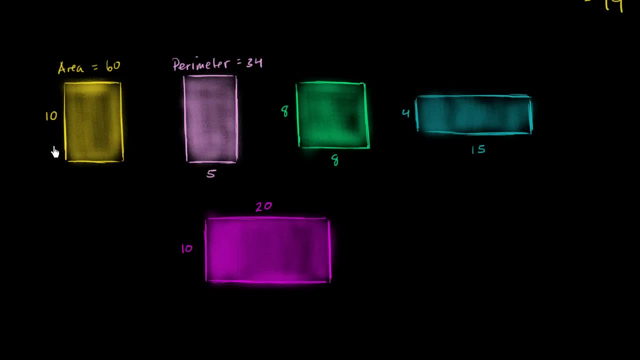 we're measuring this 10 in, So what I want you to do is now pause this video And based on the information given on these other rectangles, so in some of them we give you two of their dimensions and in some of them we give you something like the perimeter- 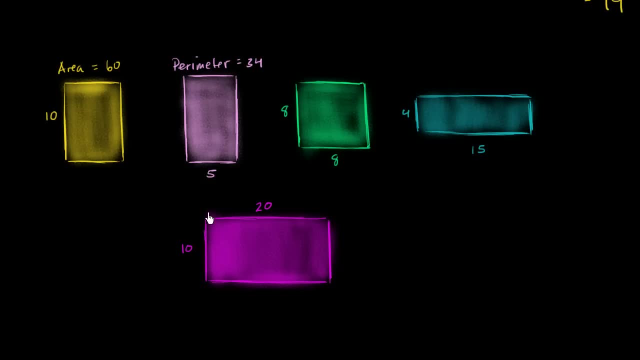 and one of the dimensions. I want you to pause the video and think about which of these rectangles, if any of them, have either the same area or the same perimeter as this yellow rectangle. So pause the video right now. Well, the best way to figure out which of these 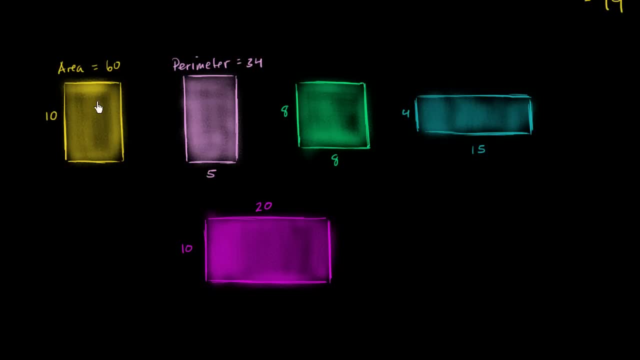 have the same area or perimeter as this original yellow rectangle is to just figure out the area and the perimeter for all of these rectangles and see which ones of them are equal, Equivalent. So we already know the area for this one, but we don't know its perimeter. 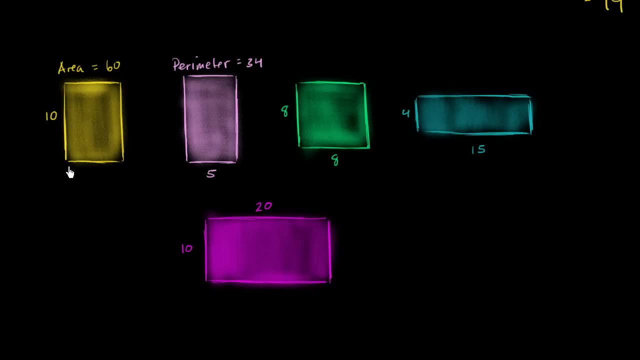 So how do we figure that out? Well, to figure out perimeter, we would need to know the lengths of all the sides. Well, if the area is 60 square units, that means the length times the width is equal to 60.. 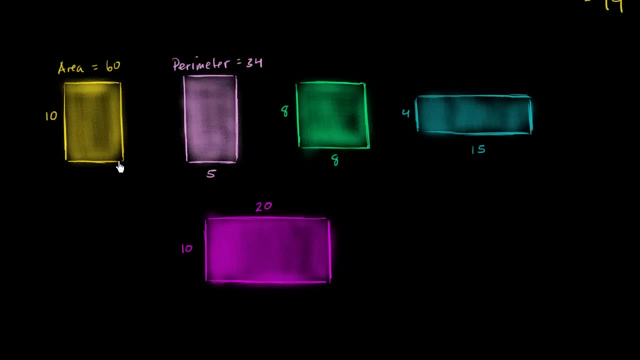 That 10 times this length or times this width right over here is going to be equal to 60.. So, 10 times what is equal to 60?? Well, 10 times 6 is equal to 60.. 10 times 6 is equal to 60 square units. 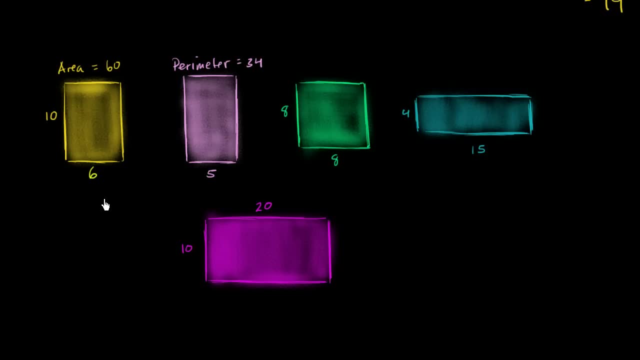 10 units times 6 units is equal to 60 square units. Fair enough, So how do we figure out the perimeter now? Well, this is a rectangle. So we know, if this length is 10, then this length must also be 10.. 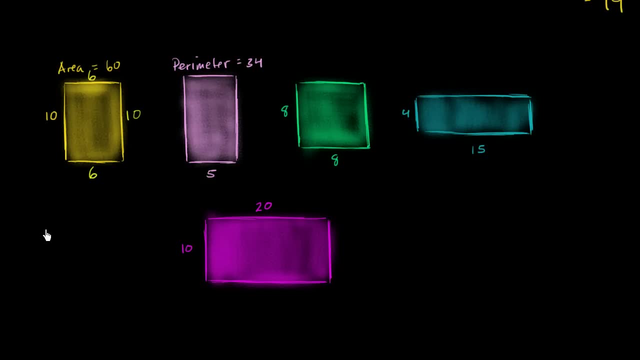 And if this width is 6,, then this width must be 6 as well. And now we can figure out the perimeter: It's 10 plus 10 plus 6 plus 6, which is 32.. So let me write that down. 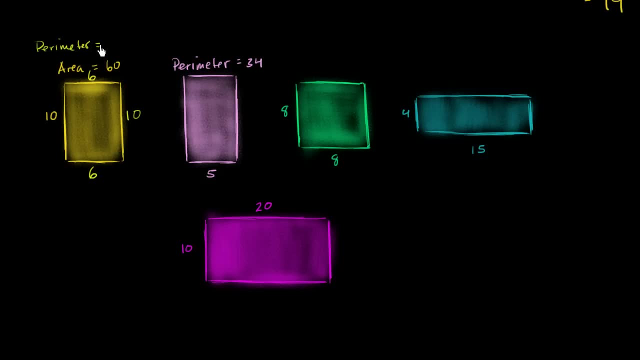 The perimeter of our original yellow rectangle is 10.. The rectangle is equal to 32.. Now let's go on to each of these other rectangles and figure out what their perimeters and their areas are. We already know the perimeter for this purple or mauve. 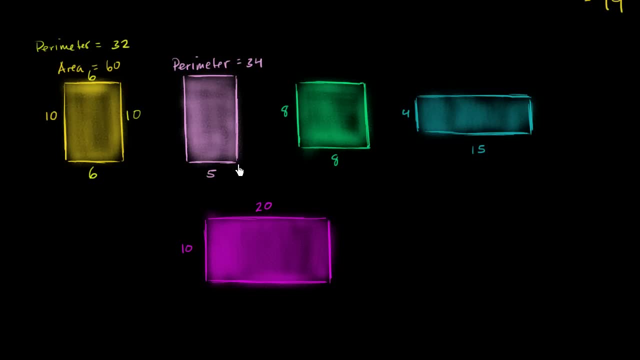 rectangle, but we need to figure out its area. In order to figure out its area, we can't just rely on this one dimension, just on its width. We have to figure out its length as well. So how do we figure that out? 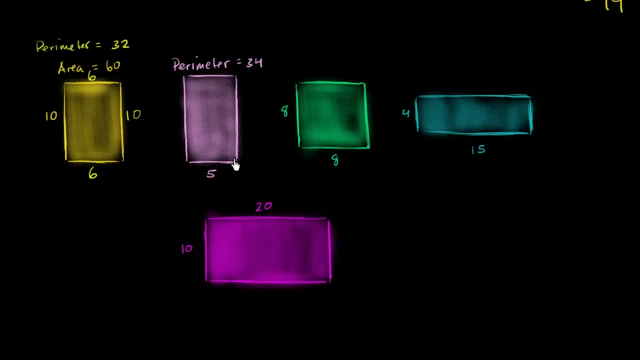 Well, one way to realize it is that the perimeter is the distance all the way around the rectangle. So what would be the distance halfway around the rectangle? So let me see if I can draw it. So what would be the distance of this side, our length? 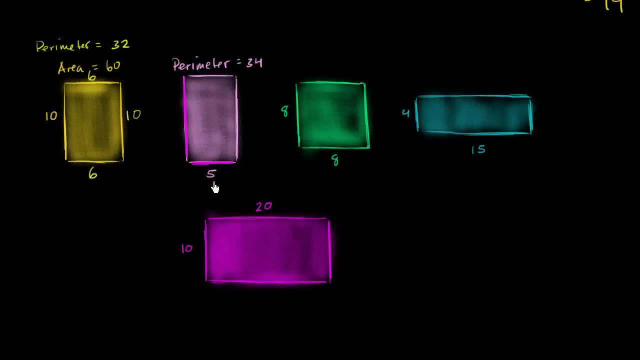 plus this side, Well, it would be half the perimeter. 5 plus something is going to be equal to half the perimeter. Remember, the perimeter is all four sides If we just took these two sides, which would be half the perimeter. 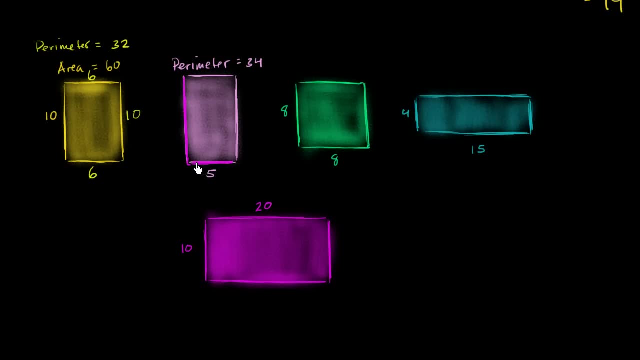 So these two sides must be equal to. when you take their sum must be equal to 17,. half the perimeter, So 5 plus what is equal to 17? 5. 5 plus this question mark is equal to 17.. 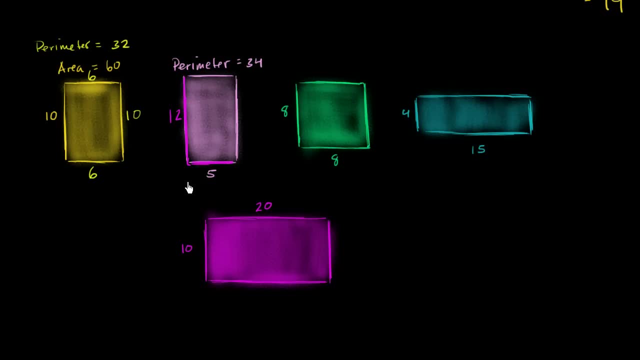 Well, 5 plus 12 is equal to 17. And you can verify this: 12 plus 5 is 17.. And then that times 2 gets us to the perimeter of 34.. Now, given that, what is the area of this figure? 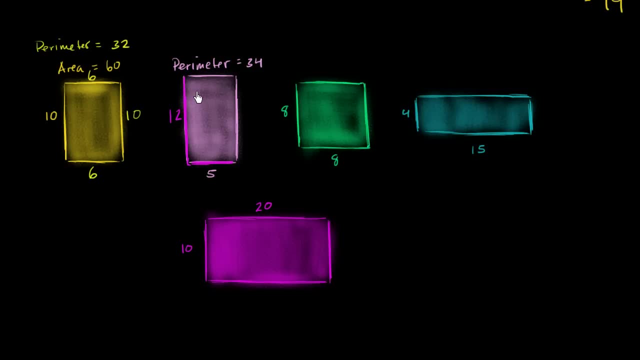 Well, the area is going to be 12 units times 5 units to get 60 square units. Area is equal to 60.. So this one right over here has the same area, different perimeter, Same area as the original, As the original yellow rectangle, different area. 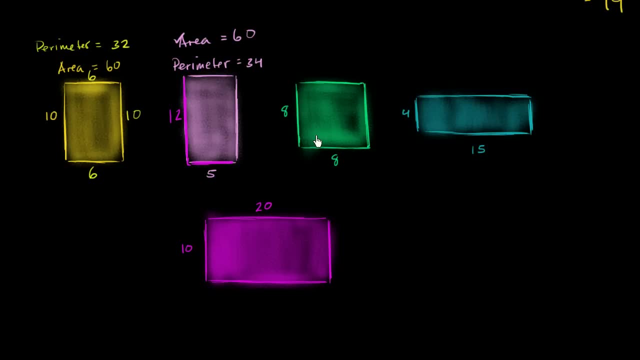 Now let's go over here. So I have- and this is not just a rectangle, this is also a square, Because I have the same length and the same width. So what's the area here? Well, for the area, I just have to multiply. 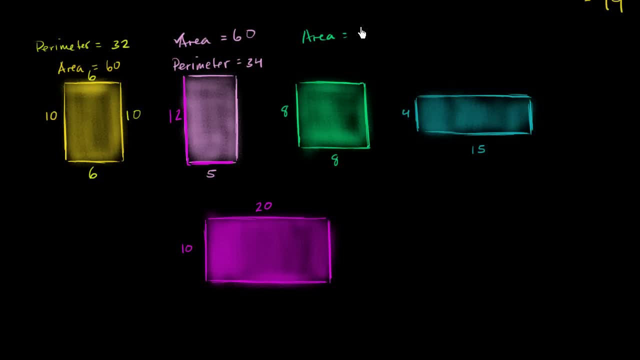 the length times the width, 8 units times 8 units is 64 square units. And what is the perimeter here? Well, these two sides are going to make up half the perimeter. If I wanted to figure out the whole one, I know this is all the perimeter. 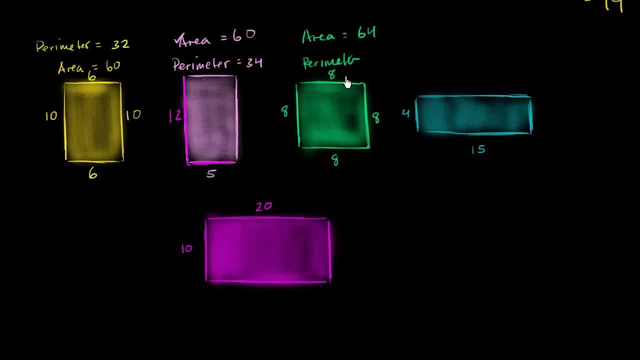 This is also 8, and this is also 8.. So the perimeter is 8 times 4.. 8 times 4 sides, which is equal to 32.. So this square right over here has a different area, but it has the same perimeter as our original yellow square. 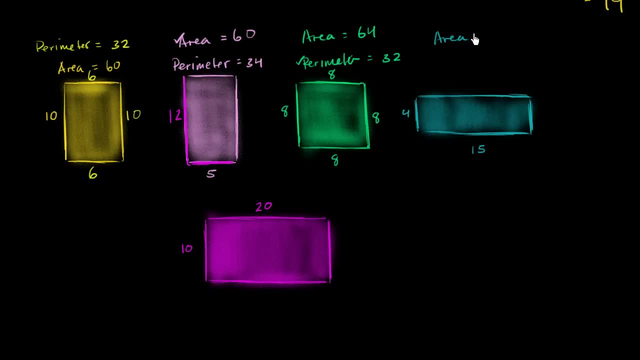 Now let's move on to this blue one. What's the area? And you're probably getting used to this: 15 units times 4 units is going to be 60 square units. And what's the perimeter? Well, it's going to be 4 plus 15, and whatever that is times 2..